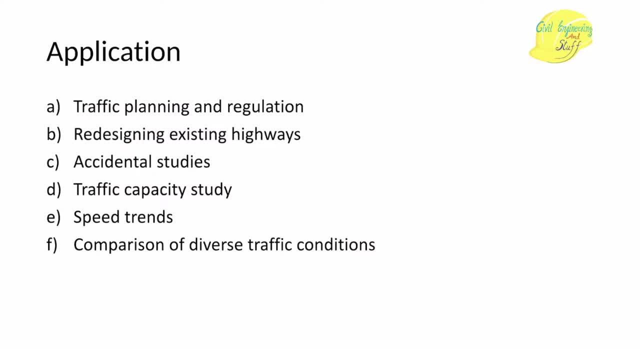 of the traffic. These are also help in redesigning the existing highways. These spot speed data are used for the accidental studies and the traffic capacity studies. By speed study we also find out the speed trend, that what is the speed bracket that has been maintained. 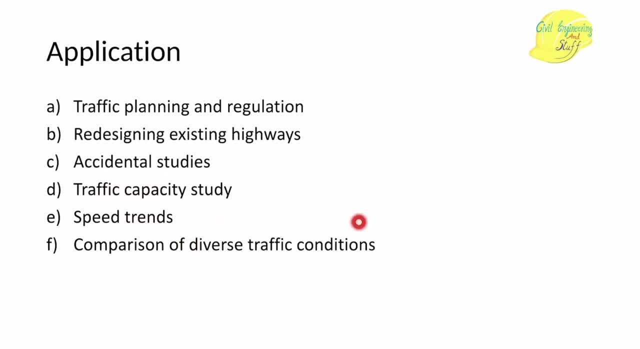 by the most of the vehicles and what are the diverse traffic conditions that are required? So what are the vehicles that are moving in that road section and what is the average speed that has been maintained by those vehicles? Now, there are number of factors that affect the speed of the vehicle. We have pavement. 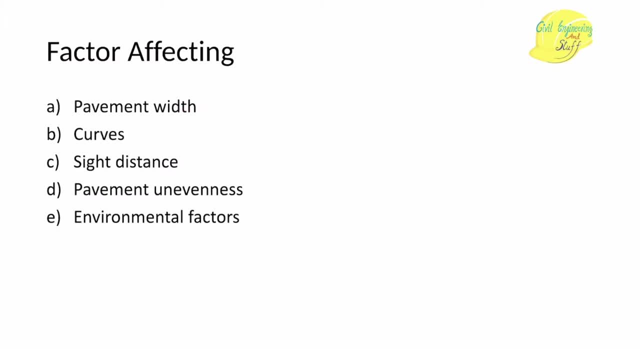 width. So wider the pavement, the more space is available for the vehicle to maintain a very high speed, and narrow width will lead to a very controlled speed of the vehicle. The second is curve. If the road section has more number of curves, then of course the speed will be less Clear. 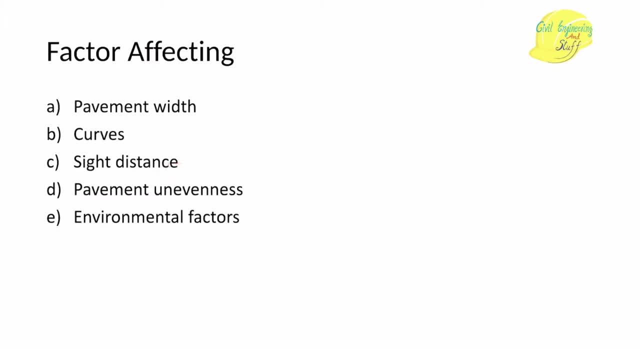 side distance promotes higher speed, and pavement unevenness leads to a very slower speed. And then we have environmental factors that affect the speed of the vehicle. So basically, if we have more rain or foggy condition, then of course the speed of the vehicle will be. 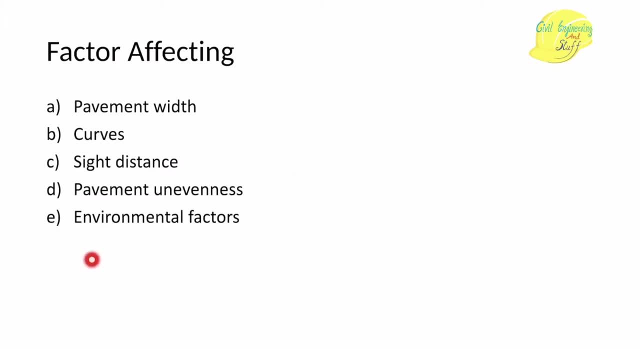 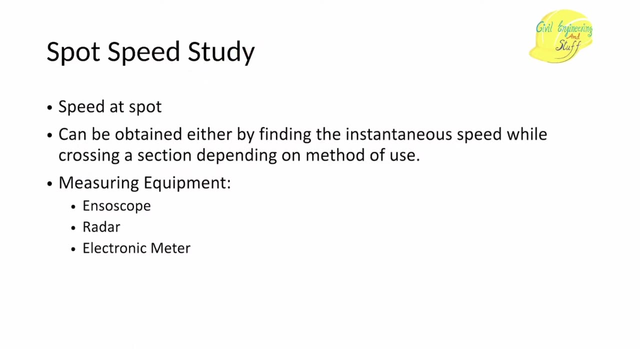 less. So these are just the common points which we all know about these, and these are factors that affect the speed of the vehicle. So now let us discuss about the spot speed. So, as we have talked about it in spot speed, we are interested in the speed of the vehicle at any spot or at any road section or at any 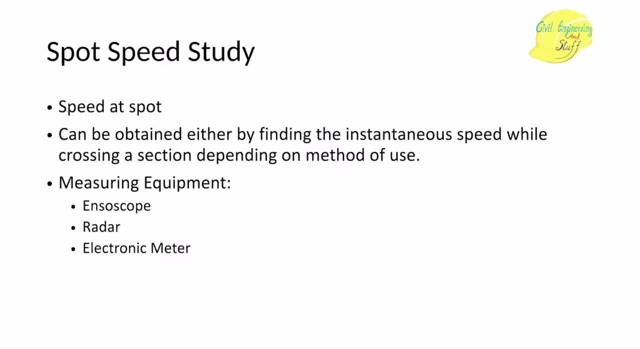 instant. Now. for that, the time mean speed can be used. the space mean speed can be used to find out the speed, the spot speed, of the vehicle. Now, there are some equipments that are used to find out the spot speed of the vehicle. So, for example, if you have a road, 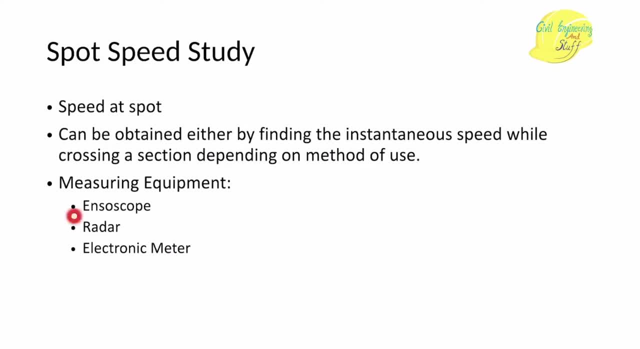 section you can find out the spot speed of the vehicle. First is an endoscope, then we have radar, then we have electronic meter. Here it should be noted that endoscope. we should remember that because many a time in competitive exam it is asked that for what? 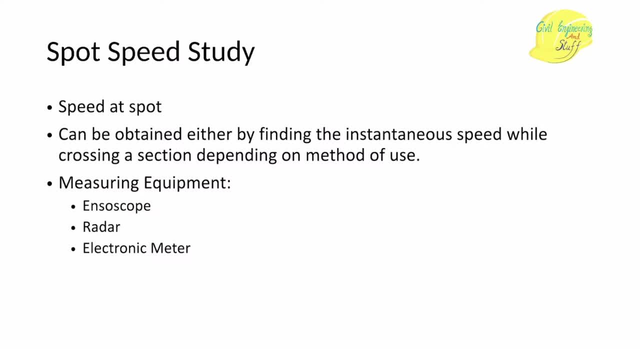 purpose the endoscope is used. So endoscope is used for the speed study and, to be specific, endoscope is used for the spot speed study. So let us discuss in brief what endoscope is. Now let's discuss an example. That's a very basic device. Suppose we have a road. 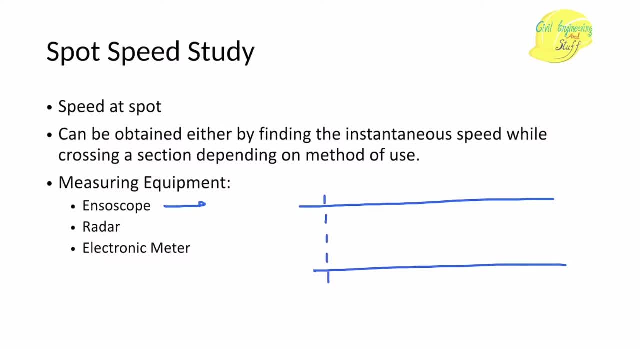 section and this road section is under observation. Of course, we know the length of this road section and at one end of the road we have the observer that is noting down the vehicle that is entering the road section, and on the other side we have an endoscope. So endoscope. 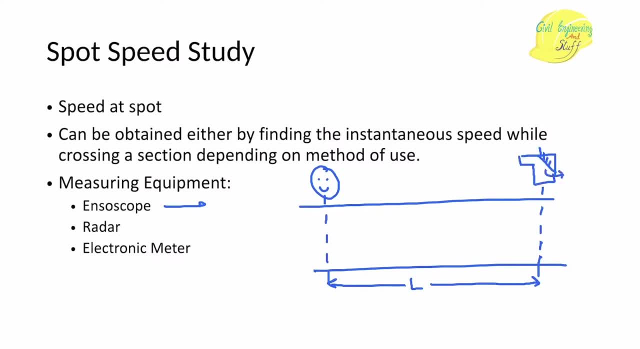 has a mirror. Second thing is the method of open-out the eyes. So this is an able-to-see endoscope. So what is endoscopy? what you do is you? This mirror enables the observer to see when the vehicle crosses this part of the road. 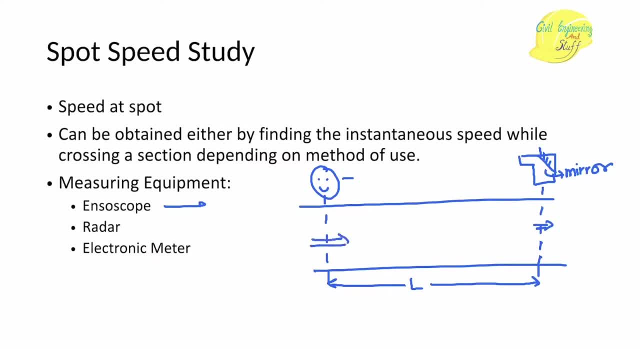 section. So as soon as the vehicle enters the road section the observer starts the stopwatch and as soon as it exits the road section the observer sees through a scope that the vehicle is exiting the road section. He stops the stopwatch and we know the length and through the stopwatch we know the time. 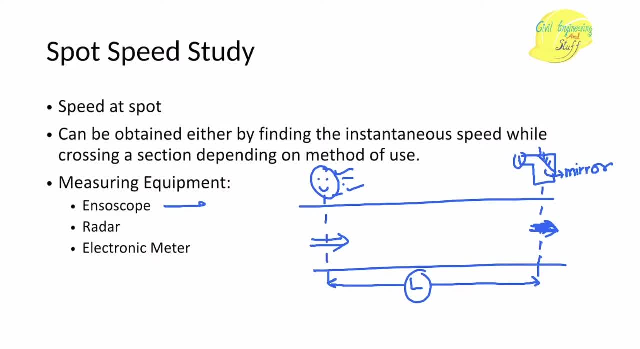 and through that we find out the speed. So it's a very basic instrument that is used to do the speed studies, And in the night we have a light source that enables to reflect the light back to the observer and through that we can carry out the speed study even at night. 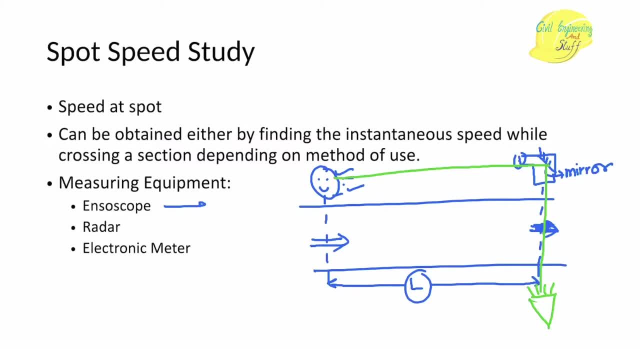 It's a very basic instrument, but then again, in many competitions it has been asked that what is the endoscope used for? So your endoscope is used for the spot speed study. Apart from that, we have a much more precise instrument. We have instruments and sensors that are used for the calculation, to find out the spot. 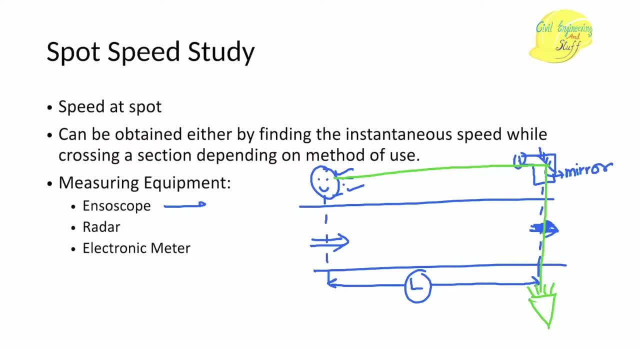 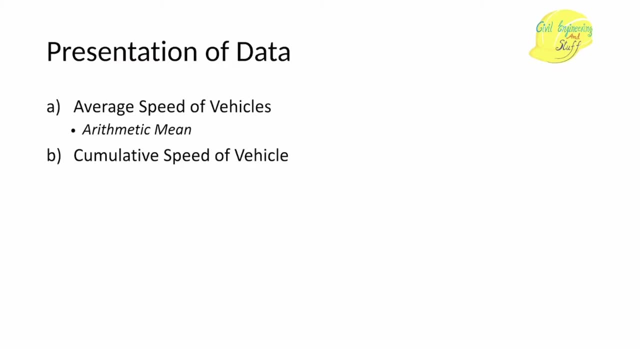 speed. We have radars, we have electronic meters and other devices that find out the speed of the vehicle at any instant and in a very much precise way. Now let us discuss the data that we have collected, how these data are represented. So your spot speed data are represented, first of all, by average speed of the vehicle. 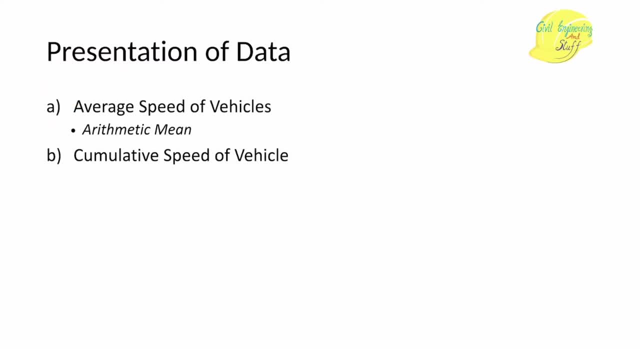 So the average speed of the vehicle is the speed of the vehicle. So the average speed of the vehicle is the speed of the vehicle. So this is the most basic way of representing the spot speed data Here. what we will do is, whatever the number of readings that we have recorded, we will. 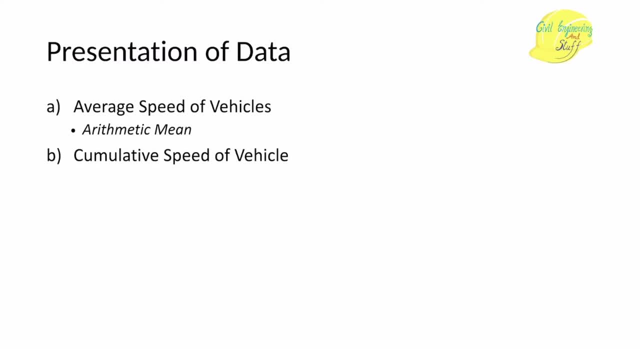 find out the average of that. So suppose, for example, we have like number of readings, We have 10 km per hour, 20 km per hour, we have 20.5 km per hour, we have 30 km per hour And of course there will be a number of readings. So we will find out the average of that. So suppose, for example, we have like number of readings, We have 10 km per hour, 20 km per hour, we have 20 km per hour, we have 30 km per hour. 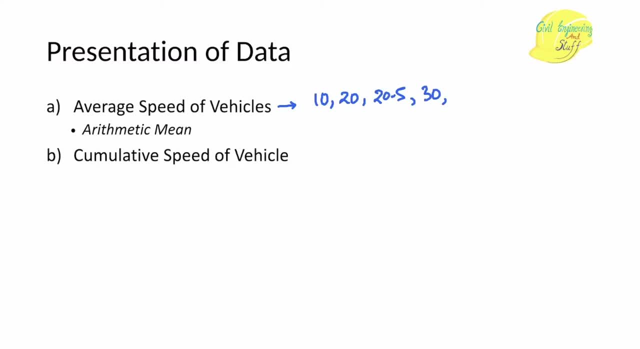 And of course there will be a number of readings And of course there will be a repetition of speed. So let us say that we again have a vehicle that is passing at 20 km per hour. Then there are vehicles that are passing at high speed. 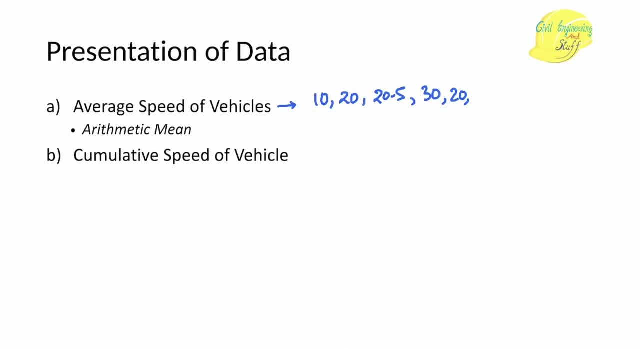 So let us say we have a vehicle that is passing at 60 km per hour, likewise 30 km per hour, 35,, 38, and again, let's say, 30 km per hour. So to find out the average speed of the vehicle, what we will do is we will sum all the data. 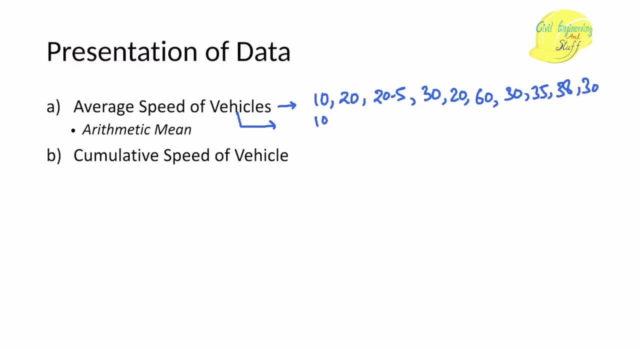 and divided by numbers of values we have. so here we have 10 values. so what we will do is 10 plus 20 plus 20.5 plus 30 plus 20, 60, 30, 35, 38 and 30 divided by 10.. so this- let's say this- comes out to be 29.3. 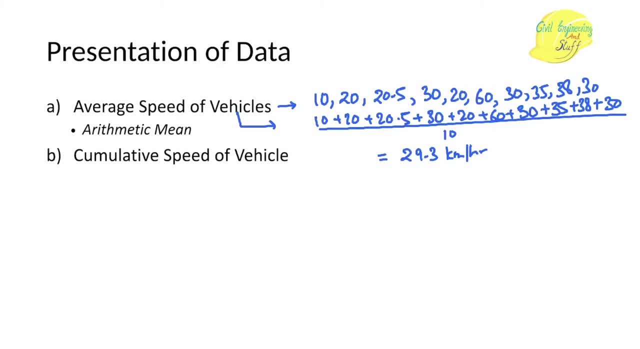 kilometer per hour. so through this we find out that the average speed that has been maintained by the vehicles that are passing through that road section is 29.3 kilometers per hour. let's round it off to like, say, 30 kilometer per hour. 29.5, 30 kilometer doesn't make much of a difference. so 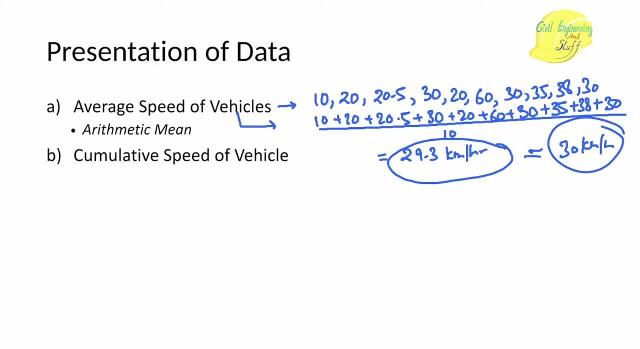 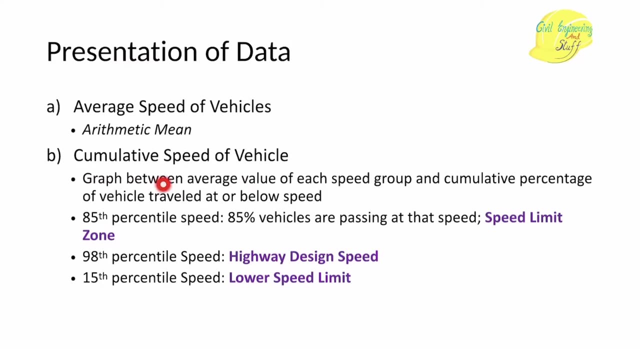 let's say the vehicle. the average speed that has been maintained by the vehicles is 30 kilometer per hour, so this is your average speed method. uh, after that we have a cumulative speed of the vehicle method to represent the spot speed datas, and here what we do is we draw a graph. okay, so? 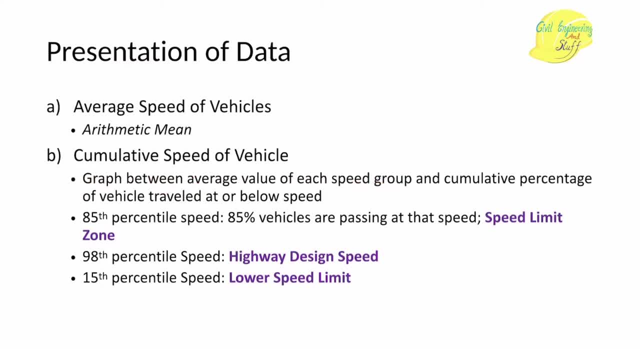 here we have a cumulative speed of the vehicle method to represent the spot speed data, and here what we do is we draw a graph. okay, so we draw a graph between the average speed group versus the uh cumulative percentage of vehicle that had traveled at at that speed or below that speed. so what we trying to achieve is we are 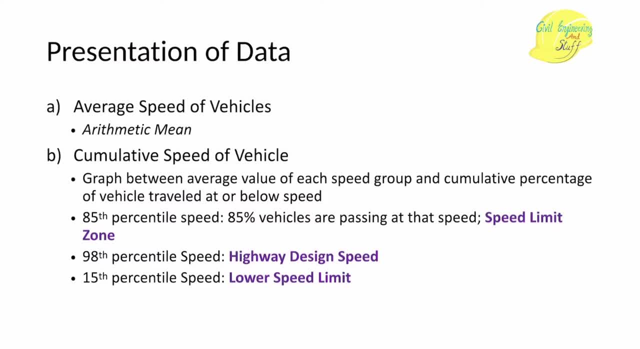 trying to find out the speed trend. so what is the percentage of the vehicle that are traveling at at that speed or below that speed? so through that we come up with certain values. so we have like 85th percentile speed, we have 98 percentile speed and we have 15 percentile speed. so your 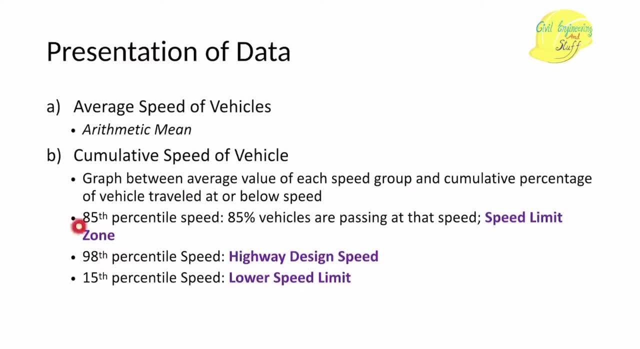 85th percentile speed denotes that the 85 percent of the vehicles were traveling either at that speed or below that speed. okay, so 85th percentile speed denotes that 85 percent of vehicles were passing at that speed or below that speed, and this 85th percentile speed is used as your speed limit. 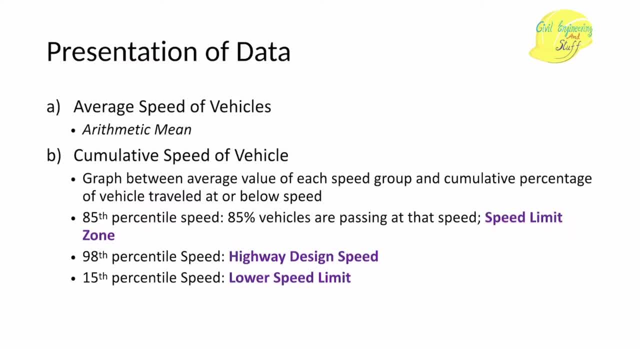 so whenever, if you are going through a road section and if you see a traffic sign that the speed limit is 60 kilometers per hour. so this speed has been defined, defined by doing doing the speed survey and through that uh, through the survey, through that survey, it has been found that uh, 85 percent of 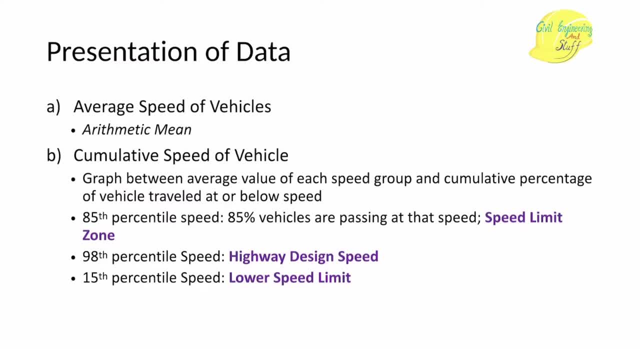 the vehicles were traveling either at 60 kilometers per hour or below that. so that's how the speed limit of the road has been decided. but then, uh, the road is designed for the 98th percentile speed. so we know that not not every vehicle will be abiding to the speed limit, right? so we have to take that. 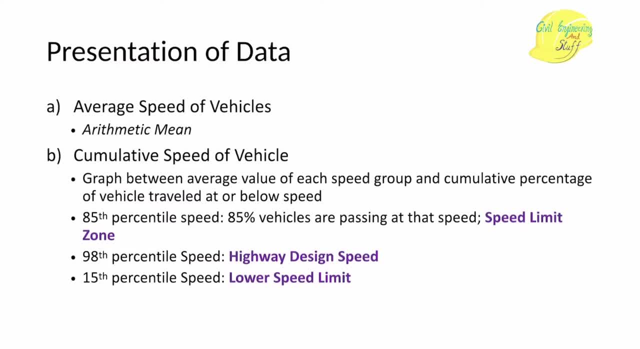 factor into account to minimize the accidents and to uh give the speed limit to the vehicle more comfort to the passengers. so for that the traffic is designed for the 90th percentile speed. so uh, let's say, during the survey time it has been observed that the uh 98 percent of the vehicles 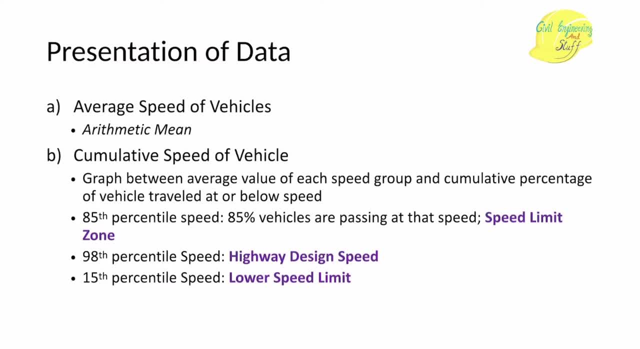 were basically traveling at the speed of, let's say, 85 kilometers per hour. okay, so the road section will be designed for the 85 kilometer per hour. that is nth percentile speed. okay, then you have a 15th percentile speed that is set as your lower speed limit. that is, this is the minimum speed. 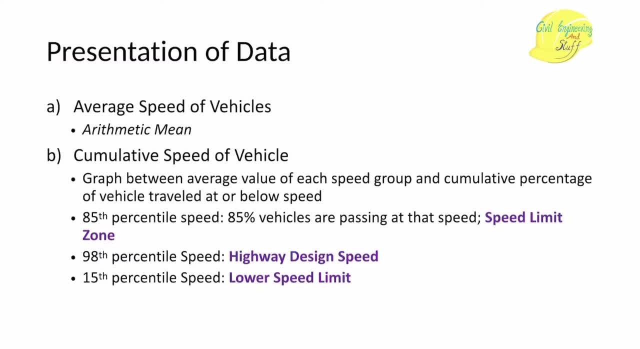 that should be maintained by the vehicle to avoid congestion. and this is 15 percentile speed, that is, uh. during a survey time, we find out that the 15 percent of the vehicles were traveling at that speed or below that speed, so let's say, 5 kilometer per hour. we have found that around 15 percent of 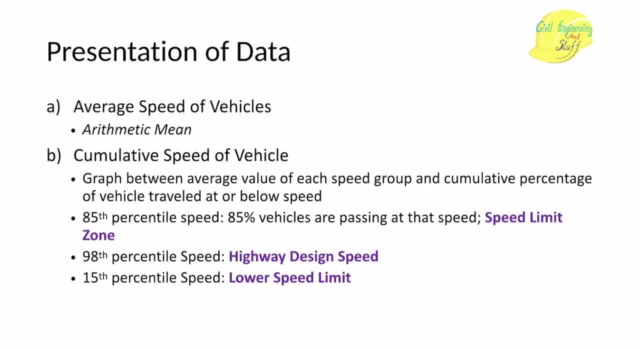 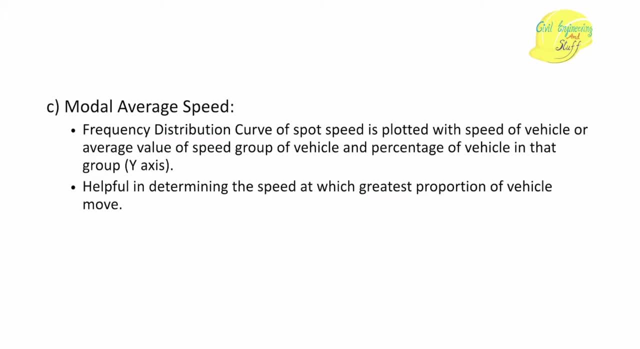 the vehicles were traveling either at 5 kilometer per hour or below that. okay, so these are the percentile speeds. the next uh way of representing the spot speed data is model average speed, so we are uh basically finding out the that speed that has been followed by most of the vehicle. 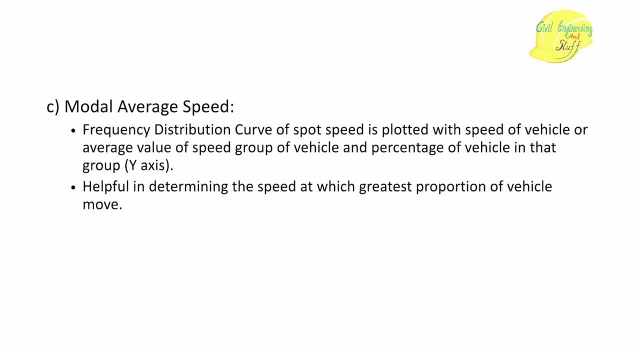 okay, so here what we do is we again draw a graph, uh, and we find out the frequency distribution graph between the speed of the vehicle and the frequency of the vehicle that were traveling at that speed. and the graph comes out to be something like this, and through that we find out the 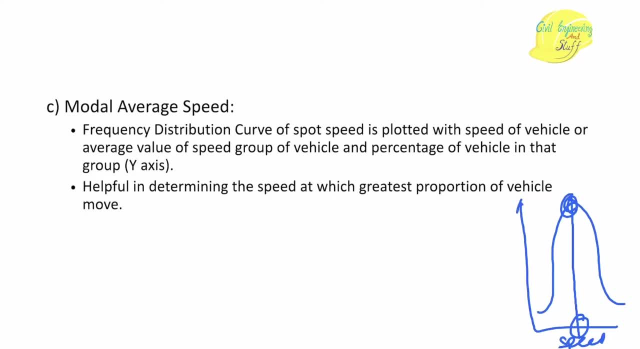 speed that has been followed by the most of the vehicles. this model average speed has to decide or find out the speed trend that has been followed by the most of the vehicle. all right, so let us discuss about this cumulative frequency method and the model average speed method through an example. so we have 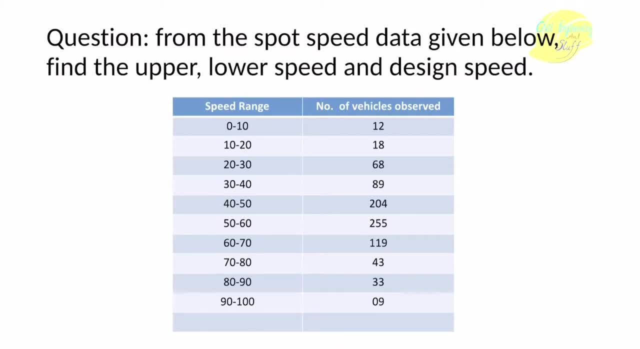 the datas through speed study and we use the same data for like for to study the cumulative method, study the model average speed method. okay, so the data will be same. so let's say, uh, the questions ask us to find out the upper limit, lower limit and the design speed limit. okay, if the question 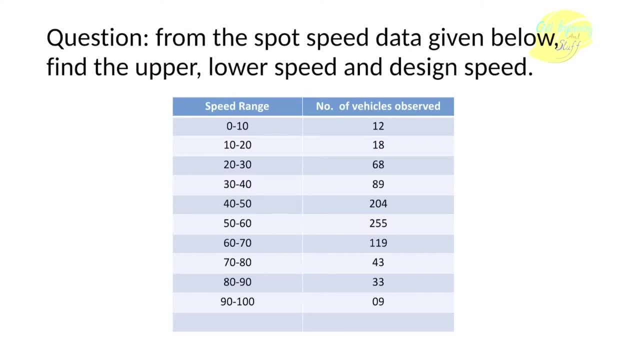 says that we have to find out the upper speed limit, we have to find out the lower speed limit and we have to find out the design speed limit, then it should be understood that we have to approach the question through the cumulative speed method, because through that only we have find out the upper limit, lower limit and design speed limit, as we have discussed. 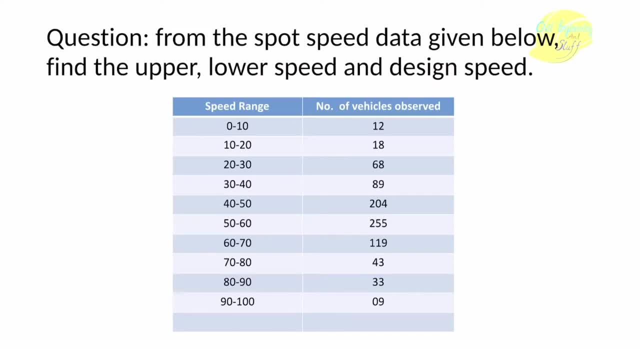 previously. okay, so, uh, we have a different speed range, so we have vehicles. uh, we have a speed range of zero to ten kilometers per hour and we have, uh, 12 vehicles that were traveling at this speed. likewise, we have 30 to 40 kilo kilometer per hour and we had 18 vehicles that were traveling. 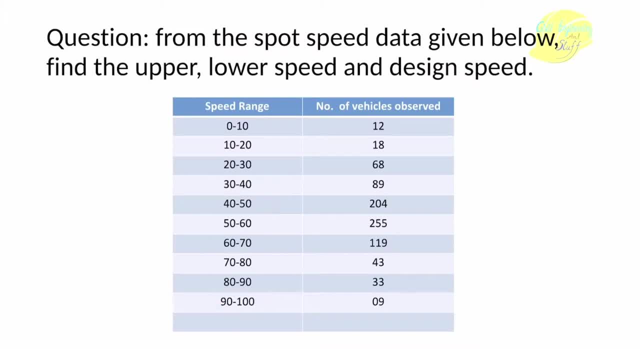 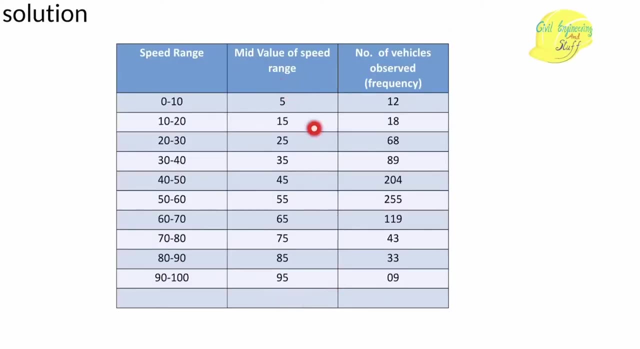 in this speed range. likewise, we have arranged those, those, uh, these datas and we have 90 to 100, we have nine vehicles that were traveling at this speed. so first thing we will do is we find, we will find out the mid-range of these. so we have find out the mid-range of that, this speed. 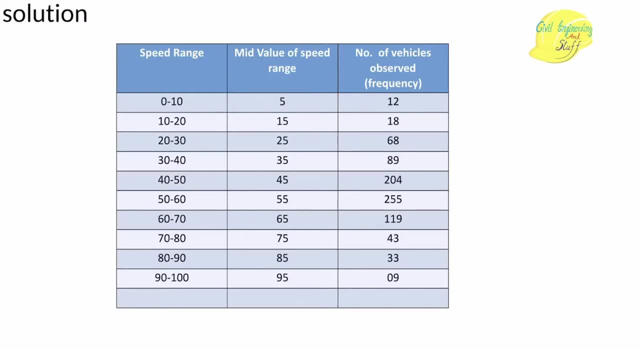 you have five. we have 12 vehicles that were traveling at five kilometer per hour. we had 18 vehicles that were traveling at 15 kilometer per hour. okay, so this is. these mid-range are nothing but 10 plus 20 divided by 2. we have 15. we have 20 plus 30. that is, 50 divided by 2, we have 25. okay. 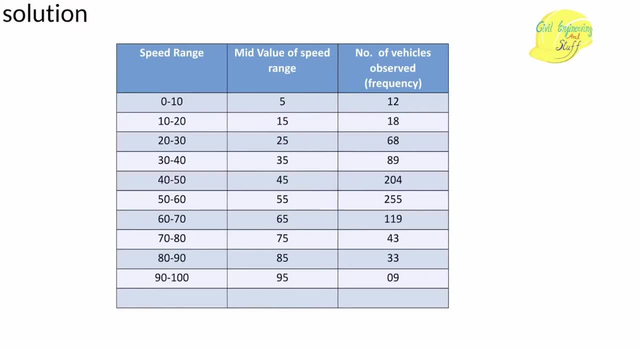 so this is how your mid-range is find out now. the next thing will be to find out the percentage frequency the vehicle of each speed. so for that, what we will do is we will to find out the percentage frequency of the vehicle that were traveling at each speed. we will, first of all, 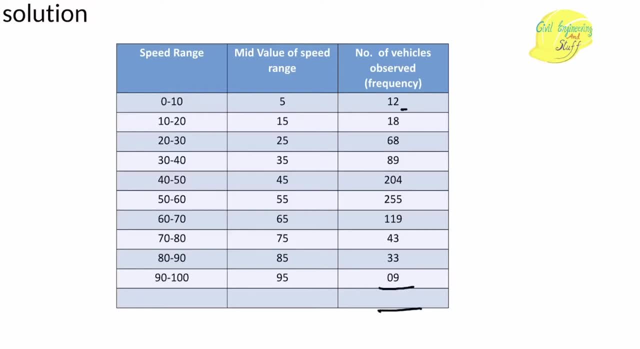 find out the summation of the overall frequency comes out to be 850. okay, so during our spot speed survey we had 850 vehicles that were passing the road section. okay, so out of these 850 vehicles, what was the proportion of these 12 vehicles? so that can be find out the percentage frequency. 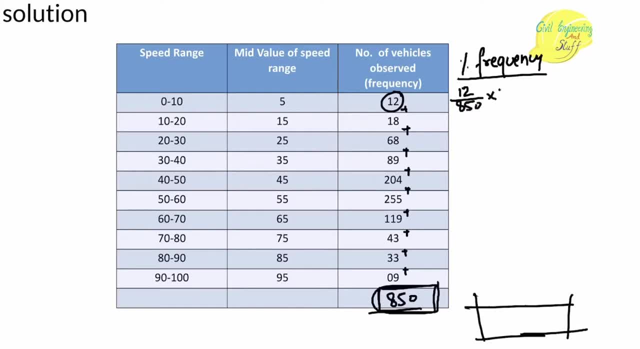 can be find out by what this 12 divided by 850 into 100, so this comes out to be 1.41. likewise, what was the percentage of the of the overall, of the total vice goes? what was the percentage of the variables that were travelling at? 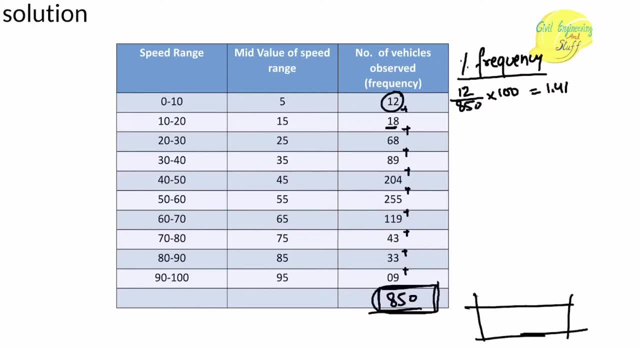 at a speed of 15 km per hour, we will find out by 870, divided by 850 into 100, so this comes out to be 2.12. will repeat the same for everything. Let's do one more. so this is how we have to find. 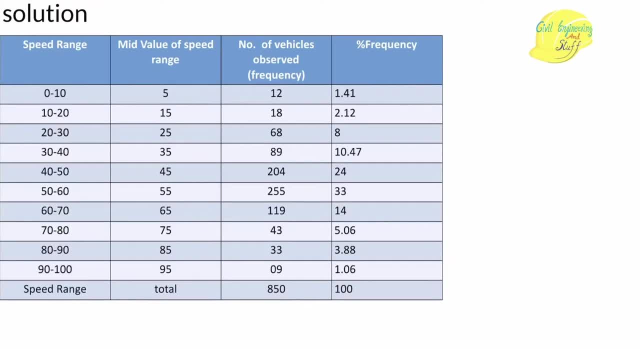 out the percentage frequency. So here we have find out the percentage frequency. Now, right now we have frequency, Now we will find out the cumulative frequency. So that is how we will get the at or below speed. So the cumulative frequency will keep adding numbers. So here, 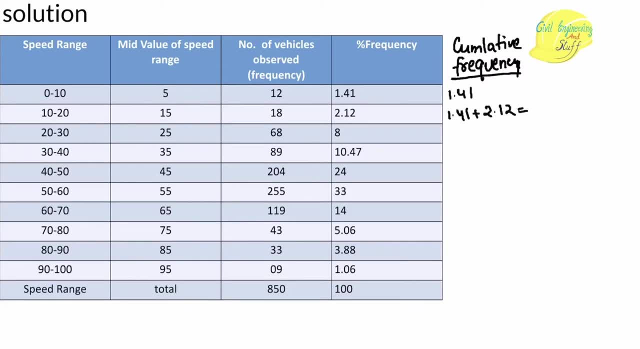 will be 1.41 plus 2.12.. So this comes out to be 3.53.. Then we have 3.53 plus 8.. This is 11.53.. Then we have 11.53 plus 10.47.. So this comes out to be 22.. Likewise, 22 plus 24, we will. 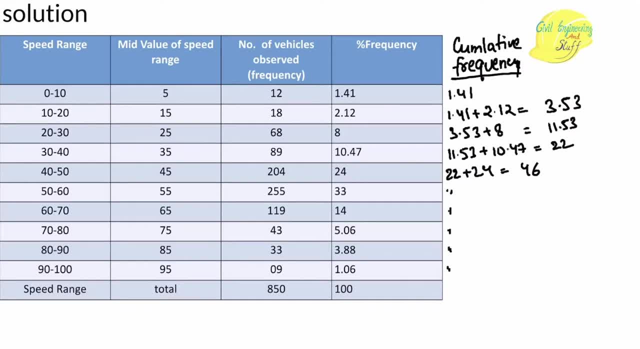 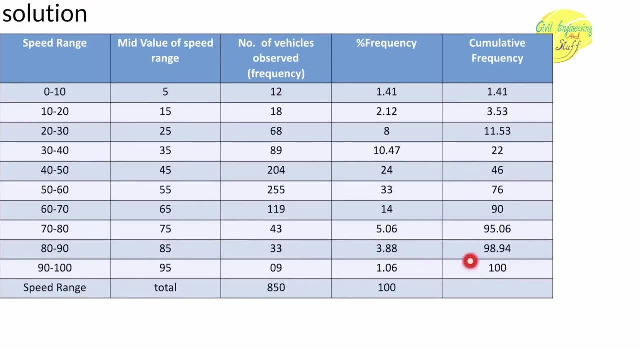 have 46.. And we will do the same for each and every data. So this comes out to be something like this: Your cumulative frequency comes out to be this: Now, what we have to do, we have to draw the graph between the speed and the cumulative frequency. 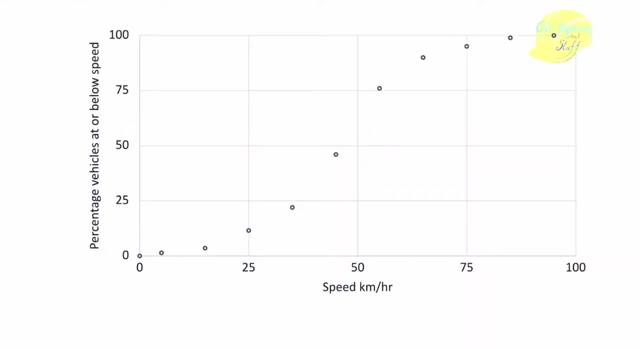 So the graph? by plotting the values, the graph looks something like this: So these are the values that we have plotted, So let's join these values. So this is the graph between the speed and the cumulative percentage. Now we have to find out the approximate speed. 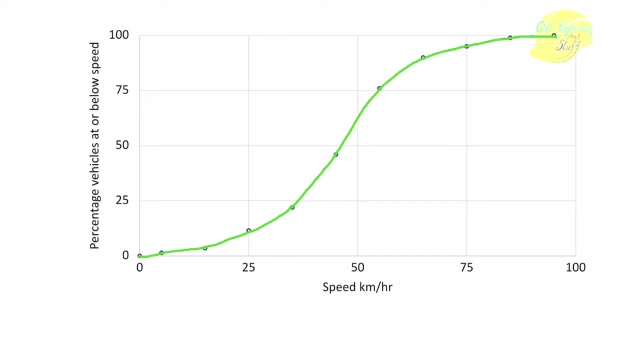 So this is the number of limits to complete a calculation. and then we have to solve the medidas. so I have an example in my graph for the prioritize нимиhes. So for example, jx2, jy2, jy2, jy3 or jy3, jx2, ie, 9, 1, 2, 3, etc. right, Jx2 got the following limits: and your jc3 wants addressing this And you have your jc2.. Then it shall know the measurement, And then jy2 has determined that it must be Modérable. It must be Modérable And it must get the jc3 to know the height, And it must get jc3 to know the height. Hola, This is the. 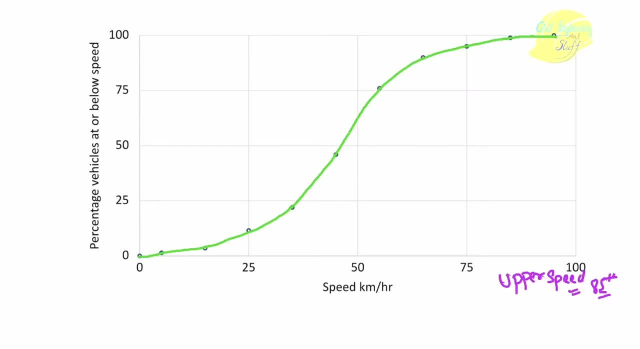 speed limit that we have Instead of my jc3,. after a calculation it starts to calculate. the milliseconds limit is 85th percentile speed. so let's say the 85th percentile speed lies somewhere here, so we'll draw here, and then we'll draw here, so this, let's say, comes out to be 60 kilometer. 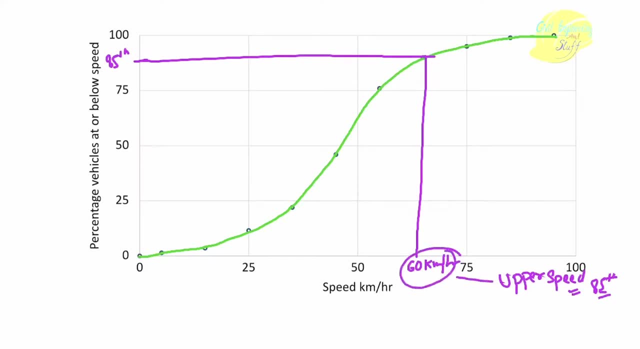 per hour. so your upper limit will be 60 kilometer per hour. next we'll find out: is design speed. so design speed is 98th percentile speed. so let's say 98th lies somewhere here, we'll draw the line and we'll draw that. so your 98th percentile speed, let's say, comes out to be: 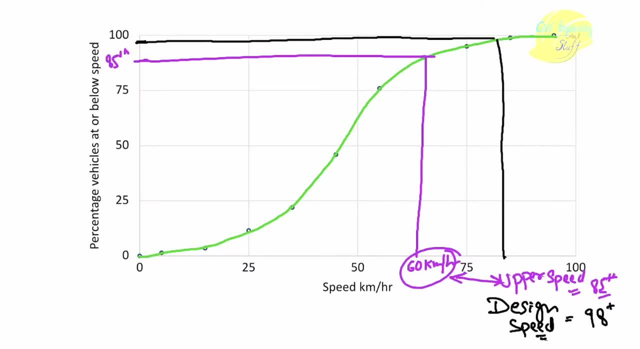 around 80. i think it is fine here. here, this is just for the example purposes. whenever you're drawing in your graph copy, make sure that each scale is well defined, right? so the here i'm just showing for the understanding purposes. but whenever you are doing the question in your graph, each value should be well defined. 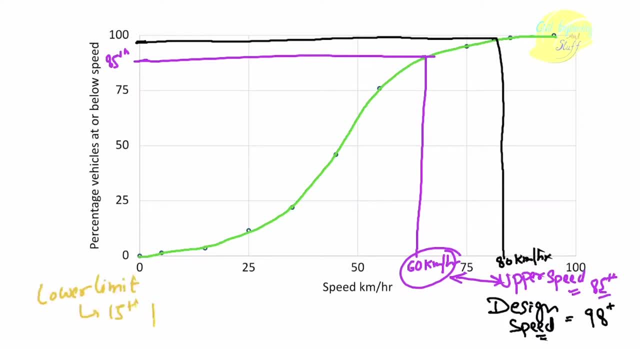 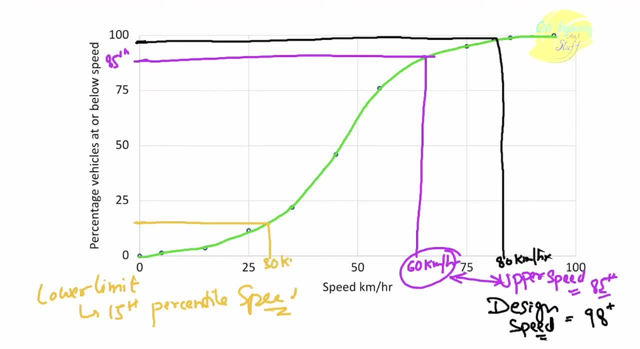 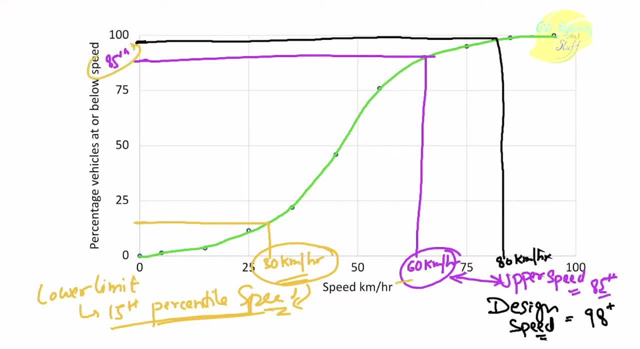 through this, we find out the 85th percentile speed, which is 60, we find out the 98th percentile speed, which comes out to be 80, and likewise we find out the 15th percentile speed. okay, so this is how cumulative speed of the. 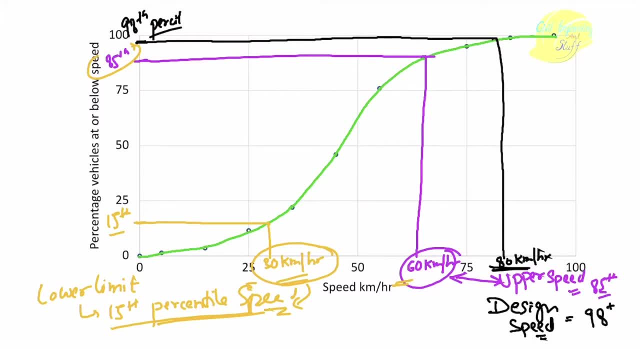 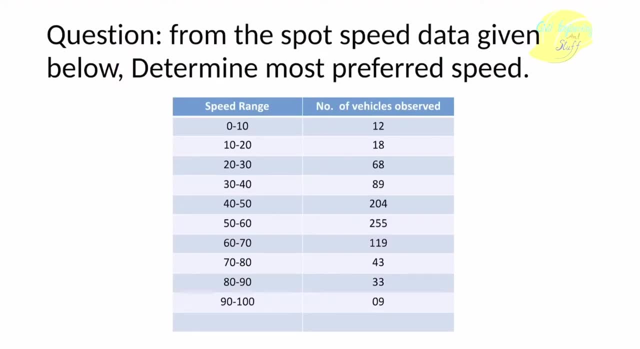 vehicle is used to find out the desired speed limits. now let us attempt the same question walking through the different method, that is, to find out the most preferred speed, and we have discussed that. when to find out the most referred speed, we use model of reach. okay, so here what we. 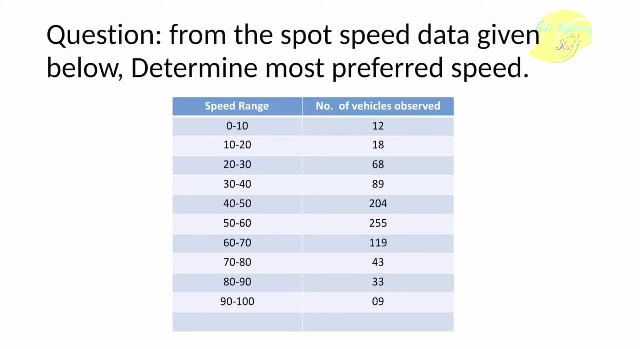 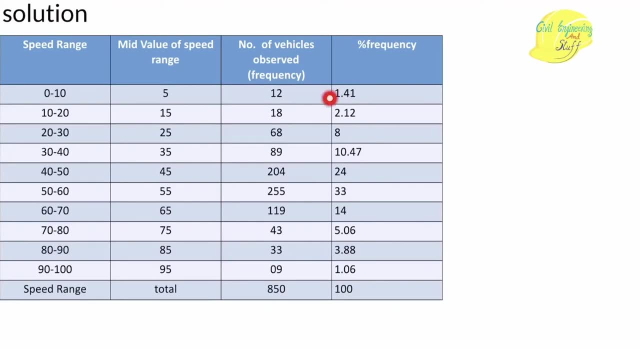 will do is, instead of percentage cumulative, we are going to use is model average. so here we will just find out the frequency of the vehicles. so we will find out the frequency of the vehicle. we have already discussed how this frequency is. find out and through this we plot these in the way in the graph. and by plotting the graphs comes out something. 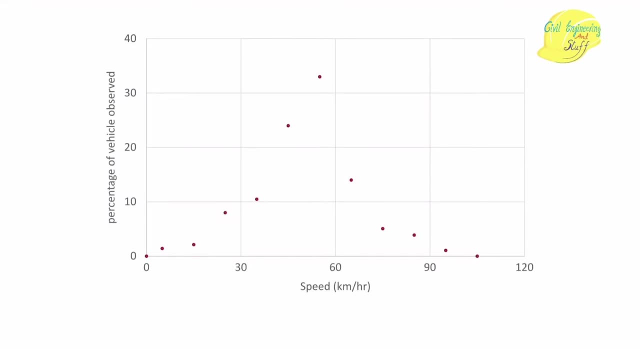 like this. so upon joining these, so we already have a very definite peak and through that we can find out. so let's say, this is 55. okay, so 55 kilometer per hour is the most preferred speed by the vehicle vehicles that were traveling through that road section. okay, so this is how the calculations 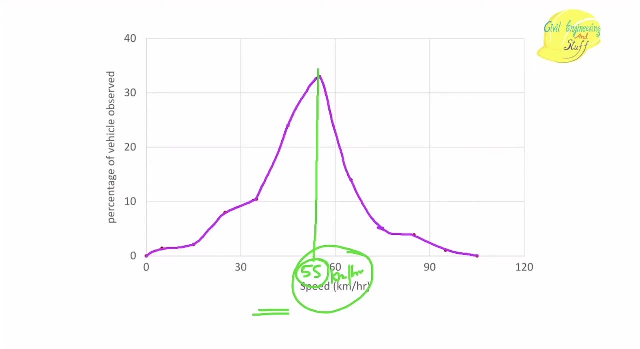 are done. so i hope this pot speed is very much clear to you and all the three methods of representation of the data and what does the technical terms that are included in these represent are very much clear to you. still, if you have any doubt and if you want me to,